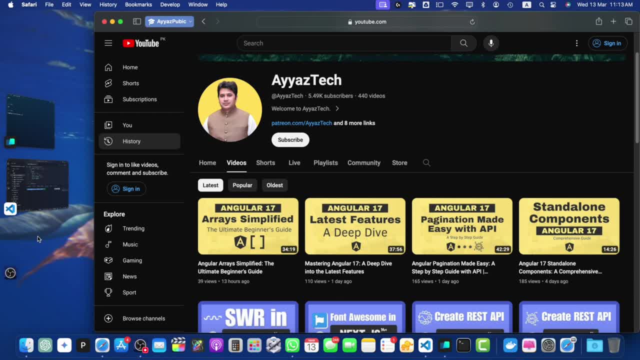 create custom HTML-like elements, loop over data to generate DOM elements and conditionally show or hide elements. The possibilities are endless. So if you are ready to master art of Angular directives and take your apps to the next level, stick around. 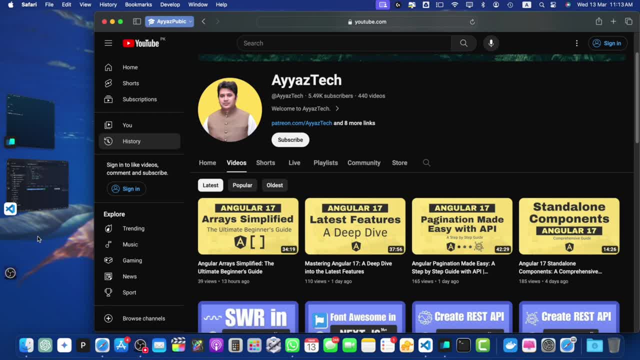 Throughout this tutorial, we will be working with the latest and greatest version, Angular 17.. We will start with built-in directives and work our way up to writing custom ones. By the way, by the end, you will be directive guru, So let's get started. 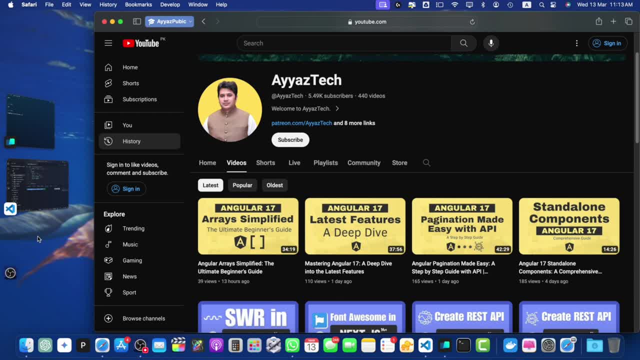 Let's dive deeper into understanding exactly what directives are in Angular. As we mentioned directives, let you extend and enhance HTML elements in the DOM. You can think of directive like a special instruction or command in your HTML that tells Angular to change or modify an element in some way when it renders to the template. 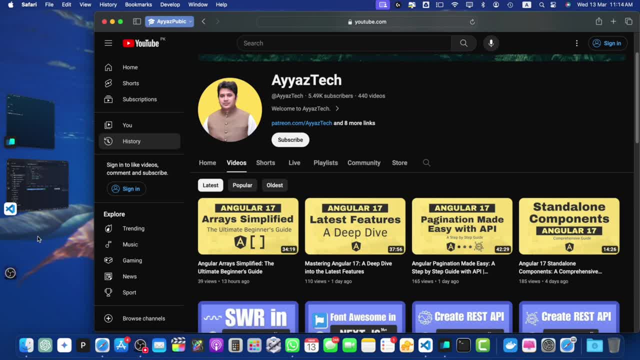 Angular provides three main types of directives that are core to how to build templates and user interfaces. So let's break each one down. First up are components. Components are directives that always have a template. They form the basic building blocks of an Angular application's user interface: Your Angular app. 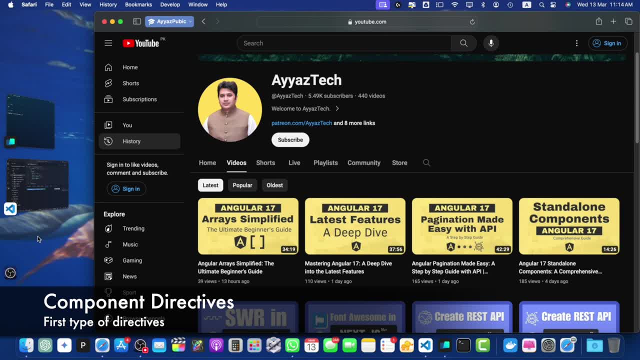 will have a root component and inside of that you will nest other sub-components to build out a full user interface. So best part of building a Angular application is that it will not have all the required components to run your application. So you need the required components to run a. 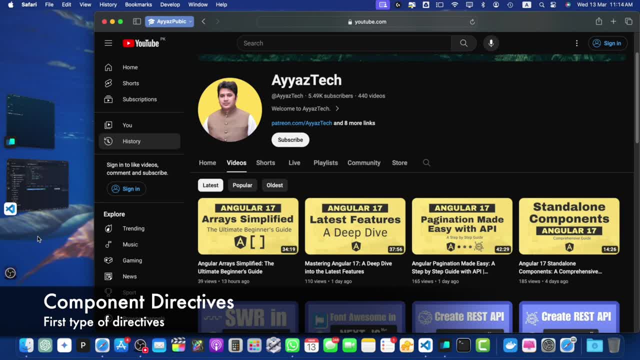 whole application. Angular provides three main types of directives that are core to how to build. So components are the most frequently used type of directive. Next are the attribute directives. Attribute directives are used to change the look or behavior of a DOM element. They are usually applied as attributes to elements. 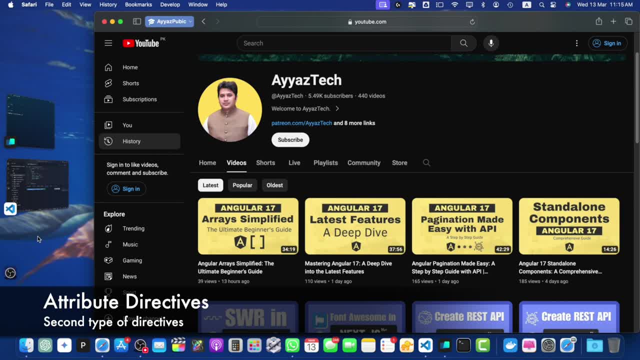 For example, Angular has built-in attribute directives like ng-class and ng-style that let you dynamically change CSS classes or styles on an element. You can also define your own custom attribute directives to encapsulate any DOM manipulation you need. Finally, we have structural directives. 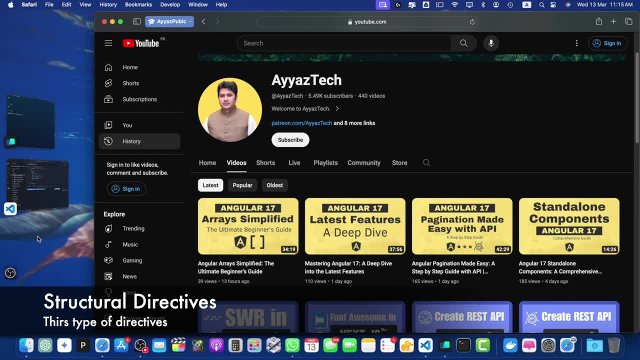 Structural directives are used to reshape structure of the DOM by adding, removing or manipulating elements. They generally operate on an element and its descendants. Angular has built-in structural directives like ng-if, ng-for and ng-switch for condition rendering elements, For conditionally rendering elements, looping over lists to generate elements and more. 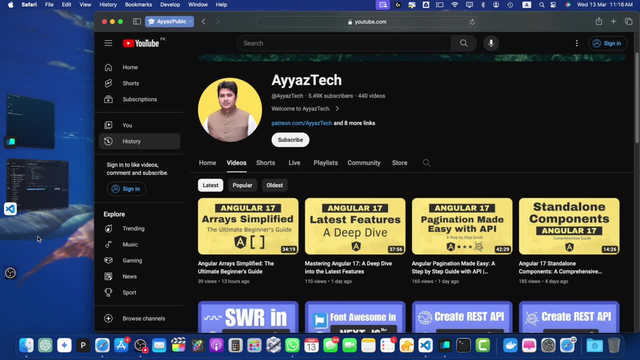 The asterisk syntax before the directive's name indicates it's a structural directive. Those are the three types of directives you will work with Angular. Through directives you get a very expressive way to write templates that go beyond plain HTML. Directives allow you to invent new HTML syntax specific to your application needs. 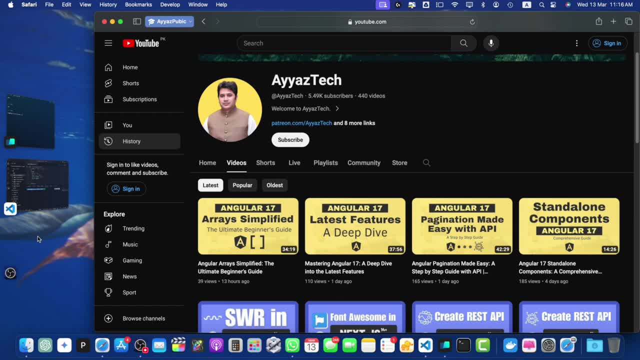 You can create directives. Directives that express complex UI patterns in a readable, declarative way, write in your templates. Moreover, directives, let you encapsulate common behavior in a reusable package. That means dry, maintainable code. You can write a directive once, then apply it anywhere. you need that functionality. 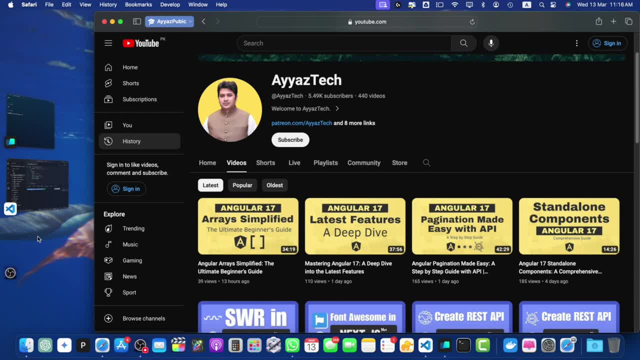 Directives are also deeply integrated into Angular's template system and work seamlessly with features like data binding. You can also create directives. You can create a property in your app that may be a file or briefcase. These are the five most important features that you need to know about your apps. 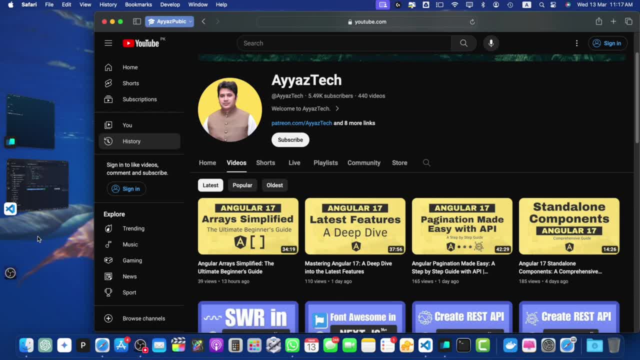 They are the following: 1. Change detection and dependency injection. That makes directives an indispensable tool in your Angular tool belt. 2. Next up, we will start looking at some of Angular's built-in directives you are likely to use on a regular basis in your own apps. 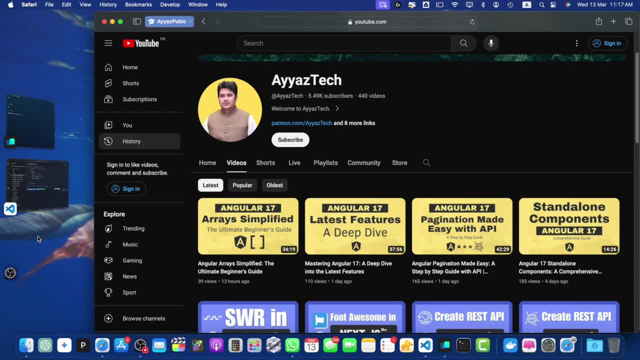 3. While Angular allows you to write your own custom directives, you don't always have to. Angular comes with a set of very useful built-in directives that you will find yourself reaching for often, So let's check out some of the most commonly used ones. 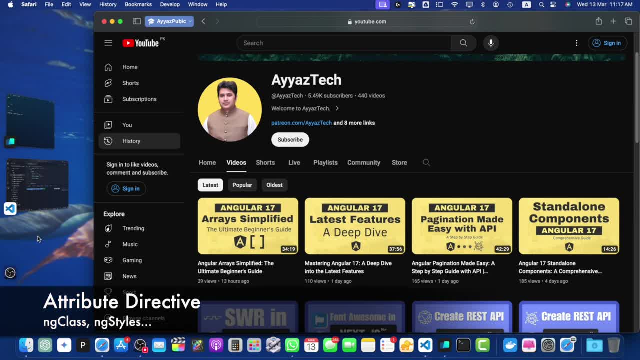 First up we have the attribute directives ng-class and ng-style. These directives let you dynamically modify, and CSS classes and inline styles on an element. With ng-class, you can pass in expression that evaluates to an object. The keys are CSS class names and the values are booleans indicating whether that class. 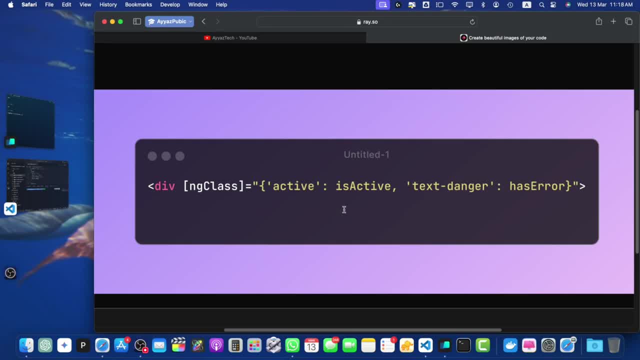 should be added or removed. So, for example, look at this code example- We have a div that has the ng-class directive on it and we are adding some classes based on some conditions. So in this case, the active class will be added if isActive is true and the text danger will. 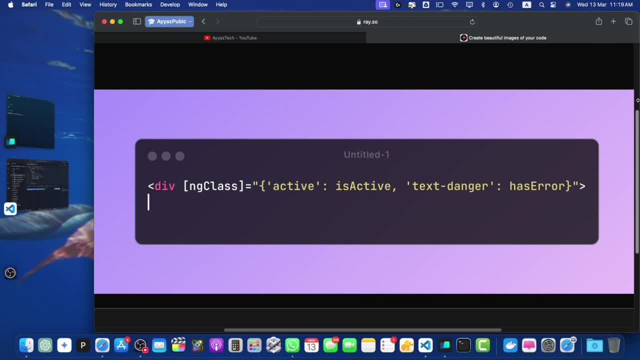 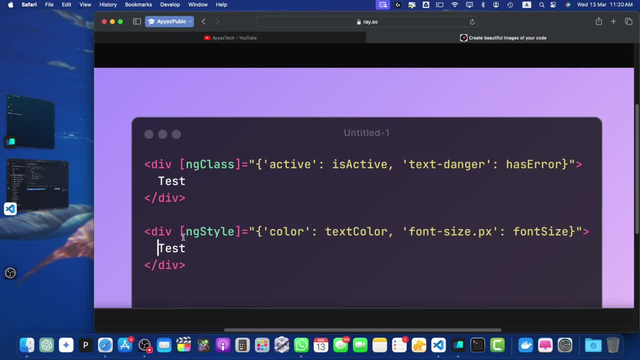 be added if hasError is true. So this is super handy for applying styles based on component state. Similarly, ng-class ng-style lets you set inline styles dynamically. You pass it an object where the keys are style names and values are style values. 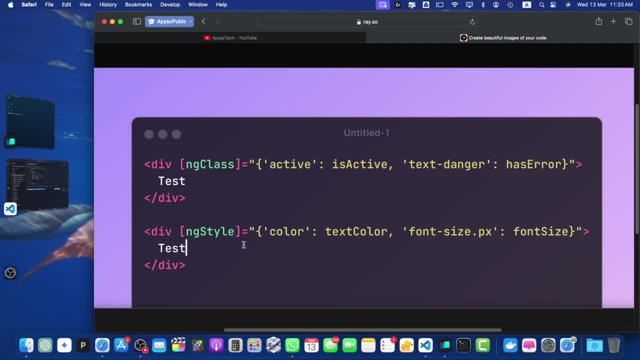 So here in this example, this sets the color and font size styles dynamically based on the component properties. So this text color and font size is coming from the angular typescript class of the component. Great for data driven styling. Next Lets look at the ng-model. 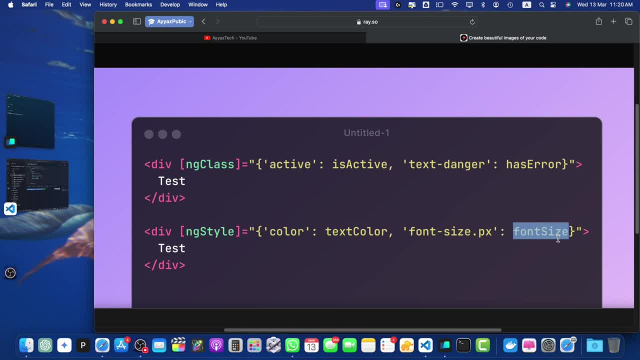 This is a special directive for two way data binding, which is mostly used with form elements like inputs, selects and text areas. With two way binding, changes to the data in your typescript class are automatically reflected in the view and user interactions with the form elements are automatically sent back. 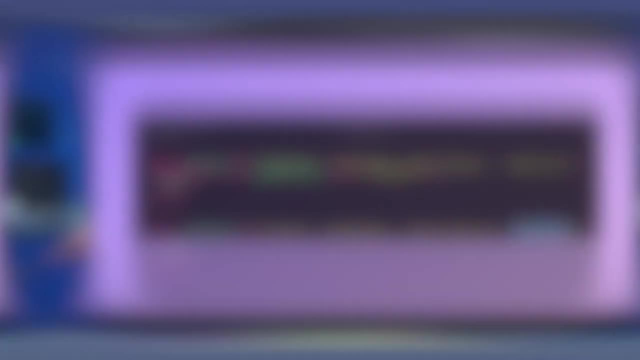 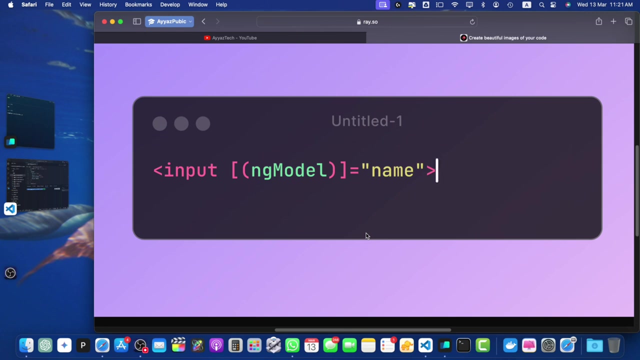 to update the data. It keeps everything in sync. So here is an example of binding an input to a property property using ng-model. Any changes the user types into this input will automatically update the name property and any changes to the name in the class will update the input's value. 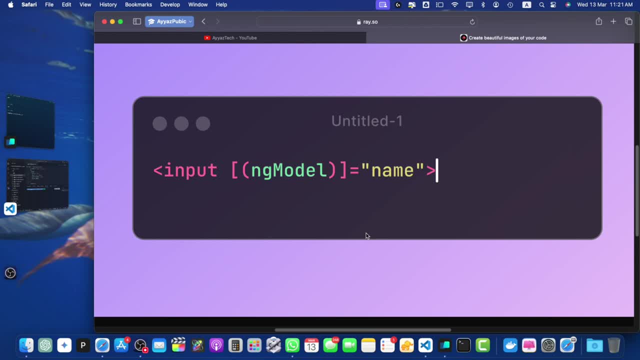 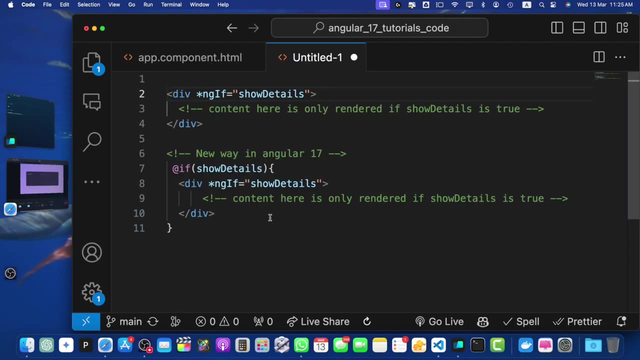 ng-model also provides features for tracking, form control, state and validity, which is super useful for form validation. Finally, lets cover the big three structural directives: ng-if, ng-for and ng-switch. So ng-if, So For conditional rendering. it will only render the element and its descendants if the expression: 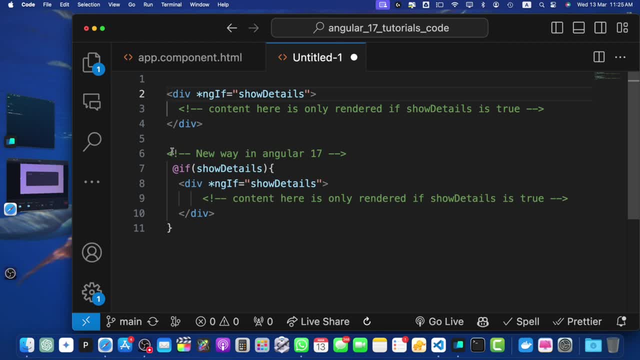 you pass it through the, So the syntax looks like this, as you can see on the screen. So this is the most popular method for using the if condition in angular. but in angular 17, this is the latest method that you can use to add the if condition you just have. 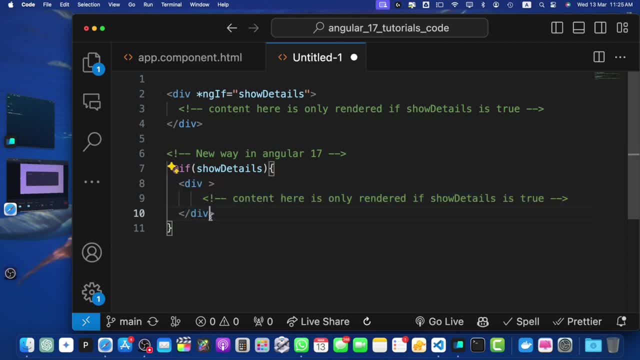 to add this and you can keep the div. So this is another way to do it. So this is an- if else- construct right in your html. Next is ng-for, Used for rendering lists of items. It repeats a template for each item in a collection. 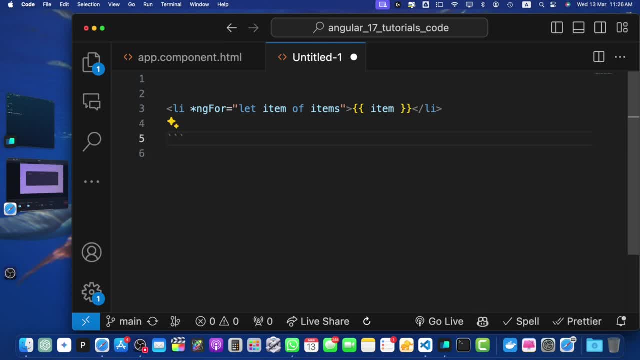 And the syntax is this. There is another latest way to do it in angular 17, that is, you just add the for loop in this way And here you will add item of items So And track itemid and then add the list within that. 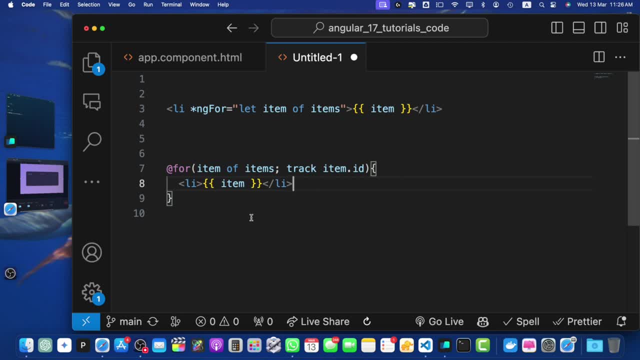 So this will loop over the items array and render an li for each one. ng-for also provides some extra micro syntax, like indexes, first last booleans and even odd properties. Lastly, we have ng-switch, which is like the switch statement for your templates. 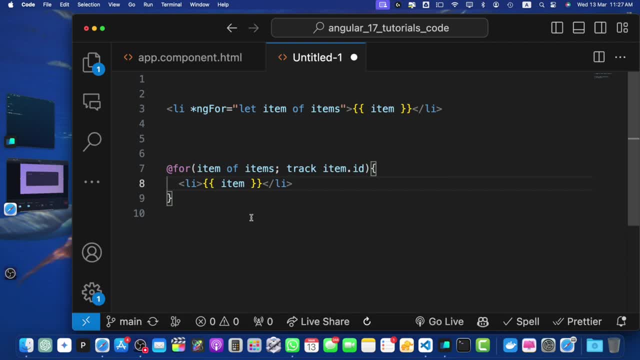 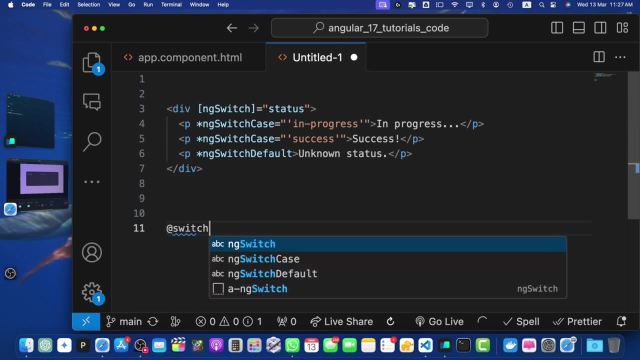 You define a switch expression And a set of possible matches and it will only render matching template. And this is how it looks like. There is also a latest way in angular 17 to add the switch. You just have to add switch in this way. 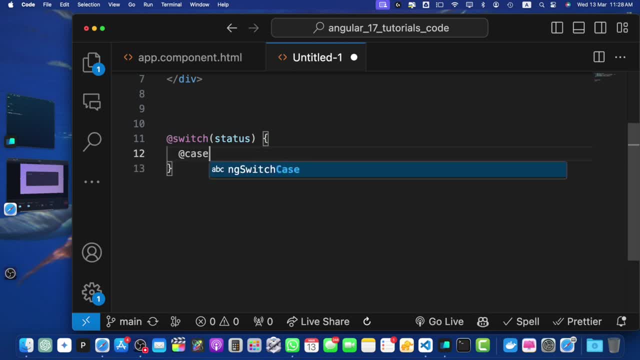 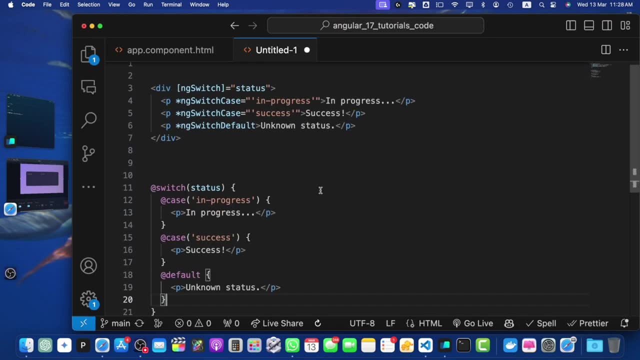 And within this we will add the case And case And finally, default. So here these are the two methods that You can use. any of these, But this one is the latest in angular 17.. So this is like an if-else chain for template fragments based on the value of status. 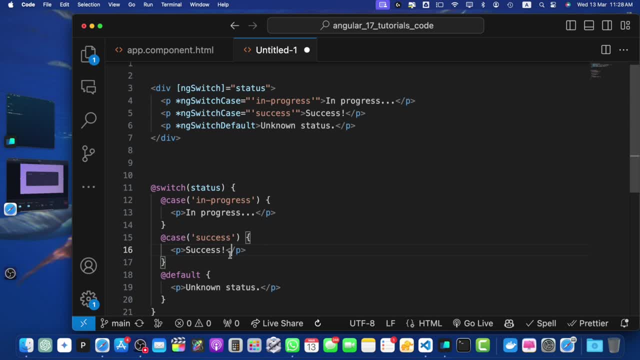 These built-in structural directives- ng-if, ng-for and ng-switch- are some of the most powerful tools for dynamically shaping the structure of your rendered HTML based on your application state and data. So that covers some of angular's most useful built-in tools. With these in your toolkit, you can create dynamic data-driven templates with conditional 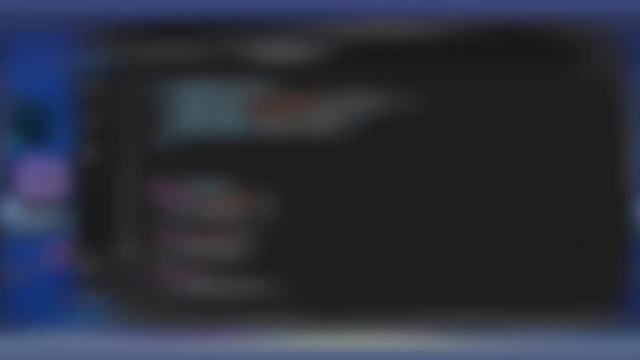 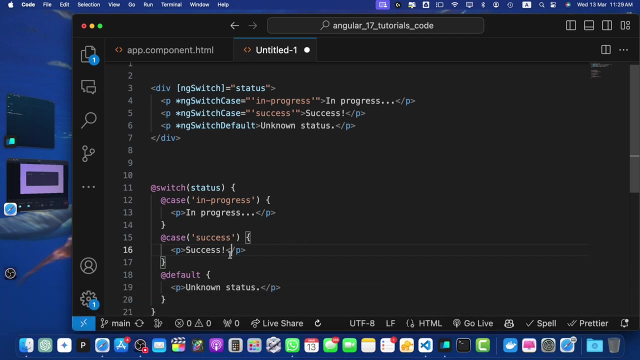 rendering, dynamic styling, list rendering and more. Next up, we will dive into writing our own custom directives. While angular's built-in directives cover a lot of common use cases, sometimes you need to encapsulate your own custom behaviours into a reusable package. 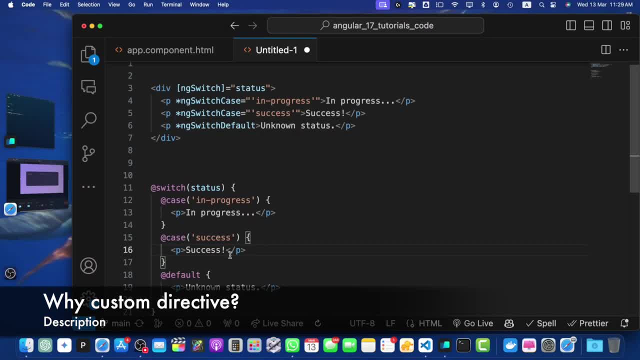 So that's where the custom directives come in. Why would you want to create a custom directive? Well, There are a few key reasons. You have some DOM, manipulation or behaviour logic that you find yourself repeating in multiple places- Directives. let you centralise that logic and reuse it via a simple directive interface. 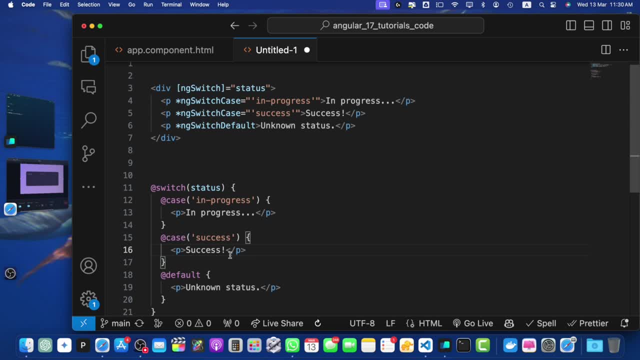 Second reason is that you need to do some complex DOM manipulation, like adding, removing multiple elements or attributes based on some state Directives provide a clean way to encapsulate this. Third reason is that you want to create a custom DSL, that is, Domain Specific Language. 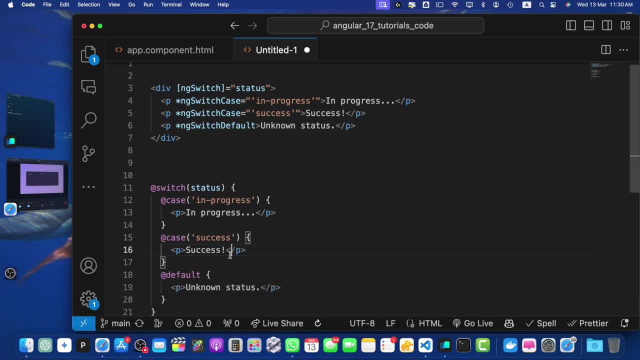 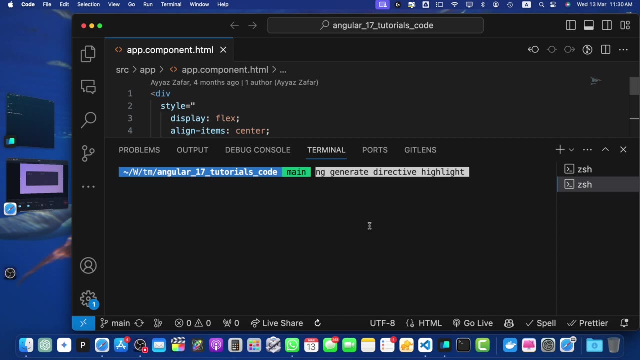 for your application's templates, Custom directives. let you extend angular's template syntax with your own abstractions. So how do we create directive? Well, angular CLI makes it easy to generate the basic skeleton. You simply need to run this command ng: generate directive and the name of the directive. 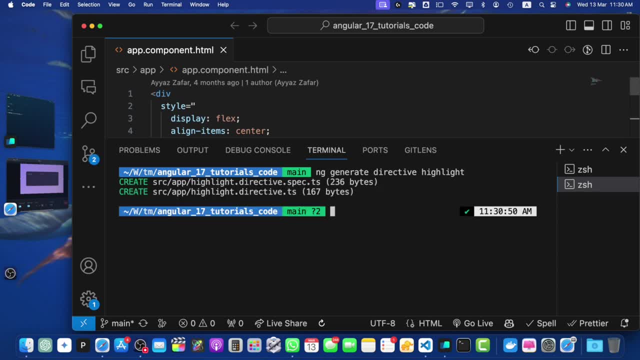 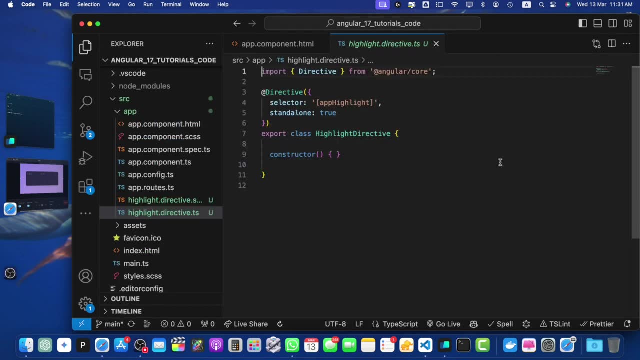 In our case, I specified the highlight, So Let's create a file called highlightdirectivets that you can see here with a basic directive structure. A directive has two key parts: the directive selector and the directive class. The selector is how you will apply the directive to the elements in your templates. 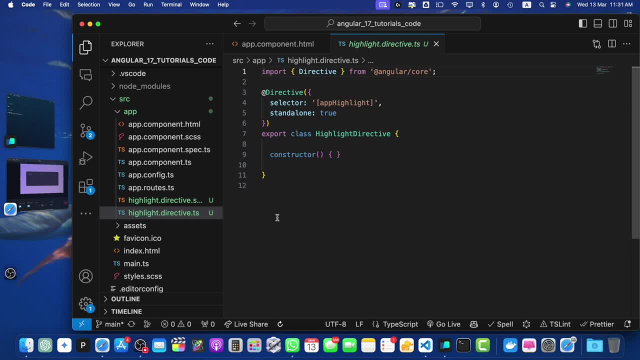 It uses a CSS selector syntax. A good convention is: use a camel case name prefix with your app prefix. So In this you can see we have the app name. In our case our app name is app, so that's why it has been fixed with app. 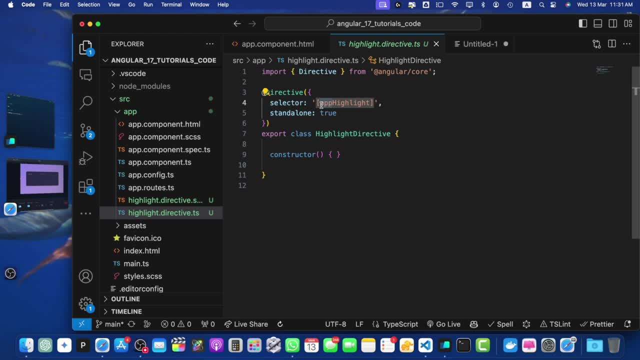 So this selector would match any element that has the app highlight attribute. The directive class is just normal typescript class, but with a directive decorator applied. This is where you will implement the directive's behavior. The class can have a constructor, which is used for dependency injection. 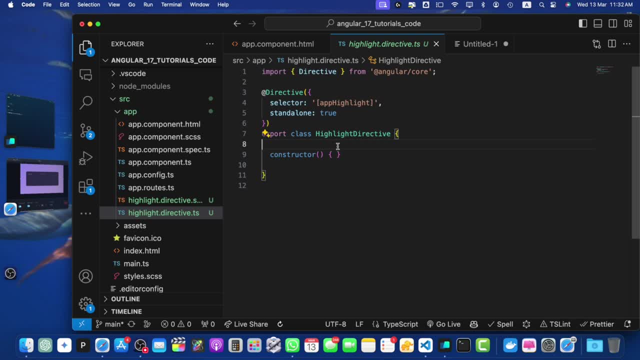 This lets you inject subtypes, So It can inject services or other dependencies that the directive needs. The class can also implement lifecycle hooks like on init and on changes. These let the directives react to changes in the host element or in the directive's. 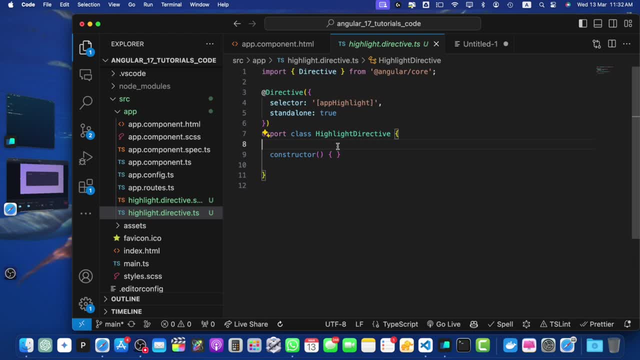 own input. Speaking of interactive with the host element, Directives have two powerful decorators for this. First one is the host binding and second one is the host listener Host bindings. This lets you bind properties of directive class to properties of the host element. 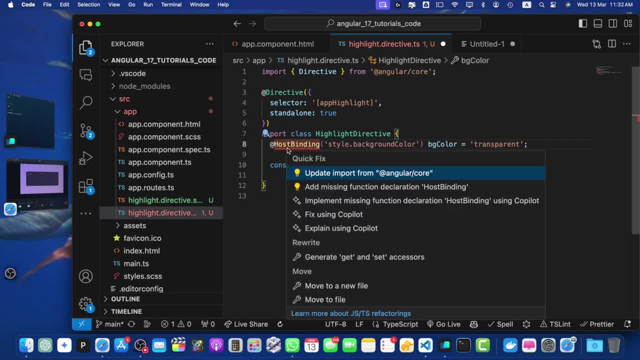 For example, This is how you will add the host binding. You have to import it from the angular core. Once you add it, You can use it. So in this case, this binds the directive's bgcolor property to the host element's background color style. 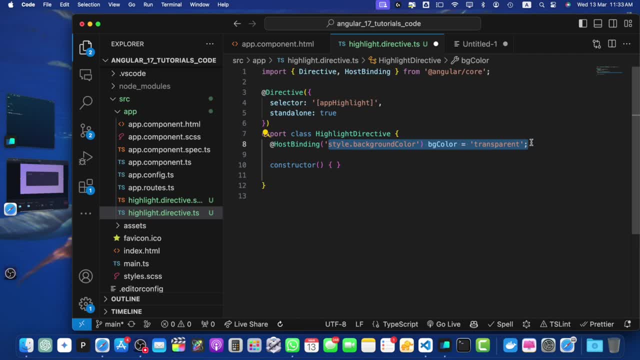 So whenever bgcolor changes, the host element's background color will update automatically. Next we have the host listener. Next we have the host listener. We have to import this as well from angular core So this listens for the mouse enter event. Next we have the host listener. that lets you listen for the events on the host element. 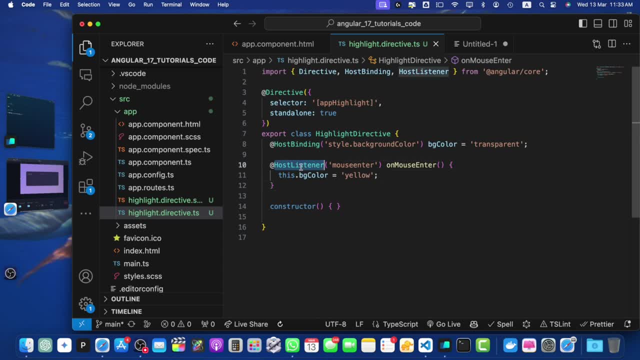 So, for example, this is the code that you can see. You have to import it as well from the angular core. So this basically listens for the mouse enter event on the host element and sets the bgcolor to yellow when it is triggered. You can also use another host listener with the name mouseLeave. 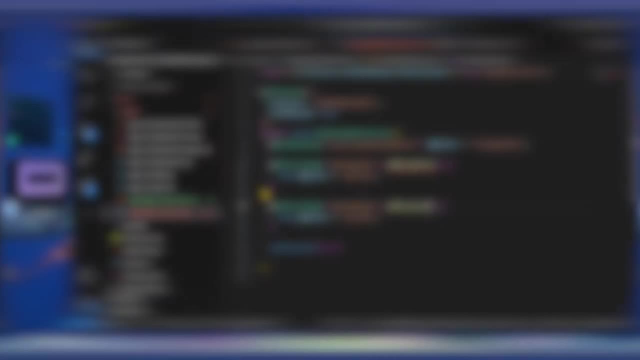 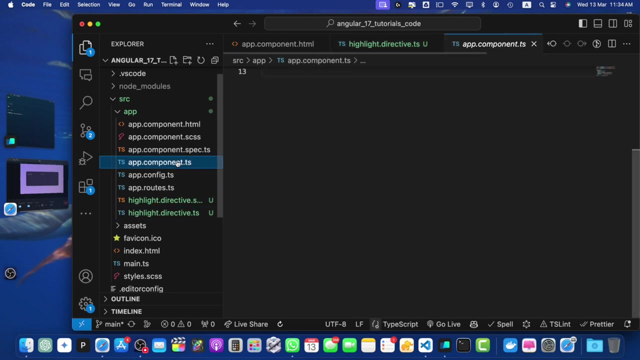 Next we have the question listener. So we have to import this as well from the angular core leave on mouse leave. so let me quickly show you how to use it. so, for example, i want to use it in the app component of ts. as i'm using angular 17, i will directly import it in the imports array. 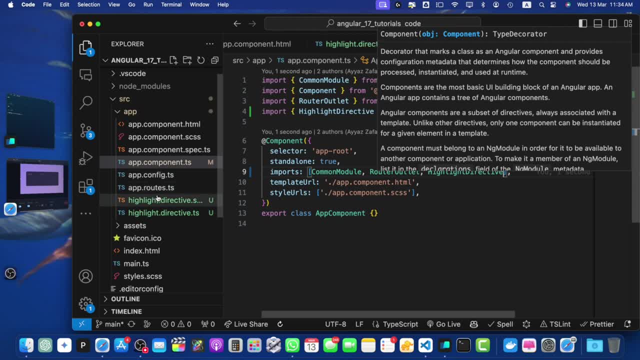 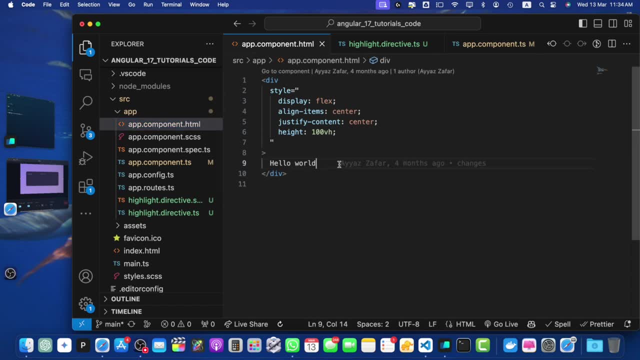 highlight directive in this way. once it is done, you are able to use it. so now let's go to the apphtml and here let me add a div, hello xyz. and here you can add app highlight in this way: now this directive is applied. now let's run our project by running the command ng serve dash o. 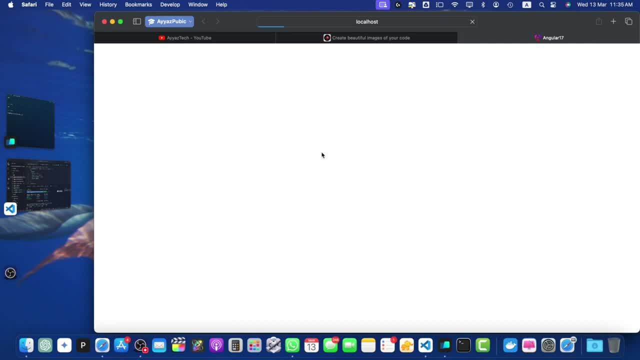 it will build and open the browser automatically so you can see that the hello xyz is visible and also the styles have been applied. so let me reload it. and right now you can see that the background color is not applied yet. but if you hover on it then the color would be applied. but if i leave my mouse, nothing. 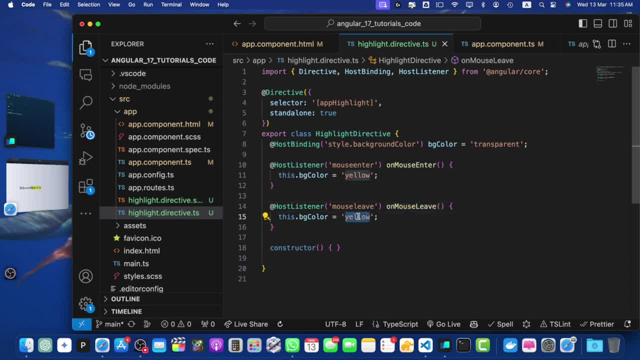 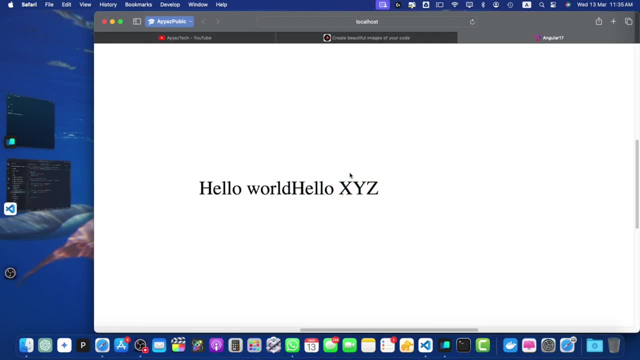 is happening because i have to correct it here. i will add the background color transparent if you leave your mouse so you can see. if i hover my mouse on it it will add the color. if i leave my mouse, then it will remove the color. so here we are adding a default background color. 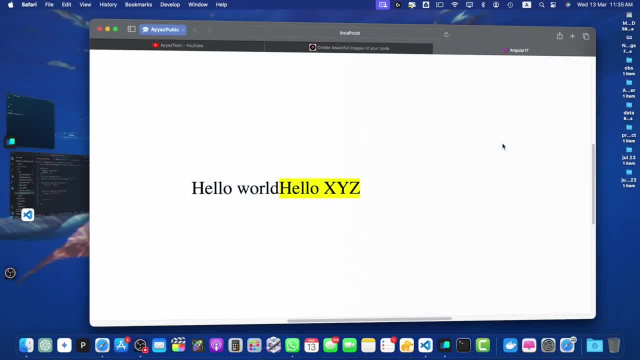 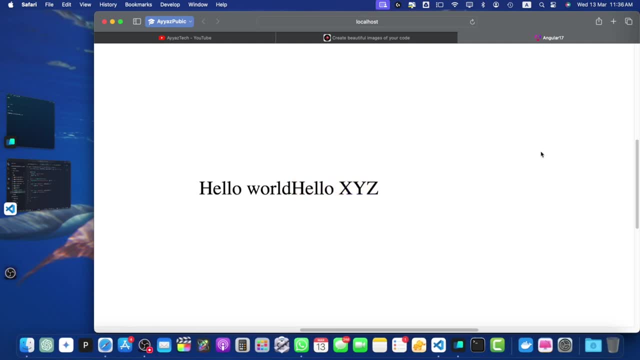 so maybe i want to add red background color. if you add it, then by default it will show the red color. if you hover, then it will show the yellow. if you leave the mouse, then it will set it to transparent. so you can see how directives let you package up this kind of reusable behavior into a neat 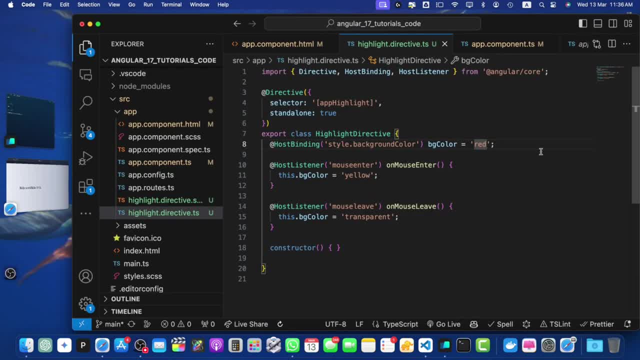 directive package and here the directive decorator, selector, host bindings and host listeners are the key ingredients in creating your own host bindings custom directive. next up, we will dive even deeper into some advanced directive techniques. so in this section we are going to dive into some advanced techniques you can use with angle directive to. 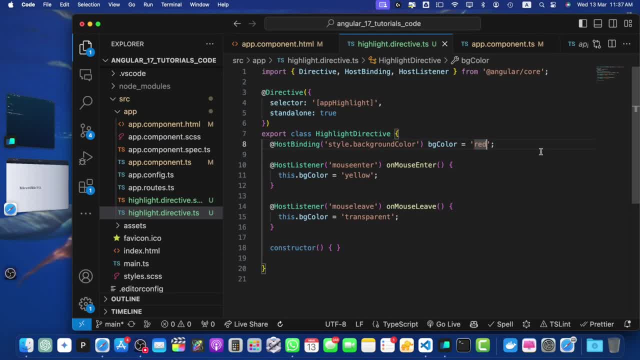 supercharge your templates even further. first up, let's talk about using directives together. did you know that you can apply the multiple directives to the same host element? this opens up some powerful possibilities. when you have multiple directives on a single element, they execute from the outermost directive to the innermost. this means, if you have directive that 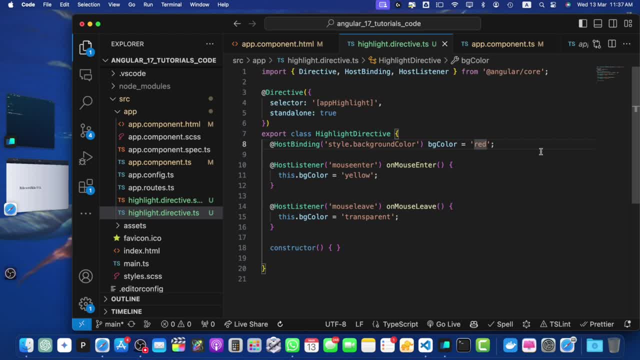 manipulates the host element itself, it will run before the directive that just deal with the elements, properties or element or events. you can use this to your advantage by creating directives that work together. for example, you might have one directive that adds a certain class to the host element and another directive that reacts to that class being present. 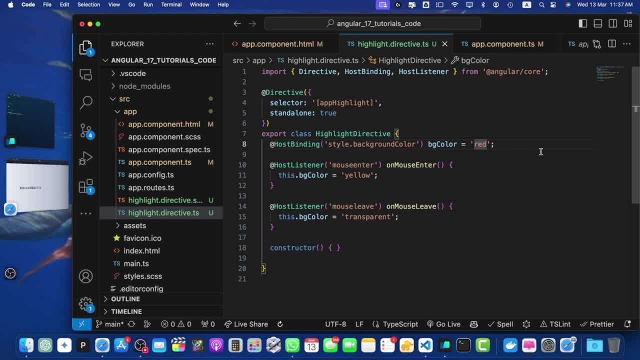 present directives can also communicate with each other- and more directory with the with each other more directly. one way is via the host element itself. directives can read and write the properties on the host that other directives can then access. another way is via a shared service. just like components, directives can inject services. this 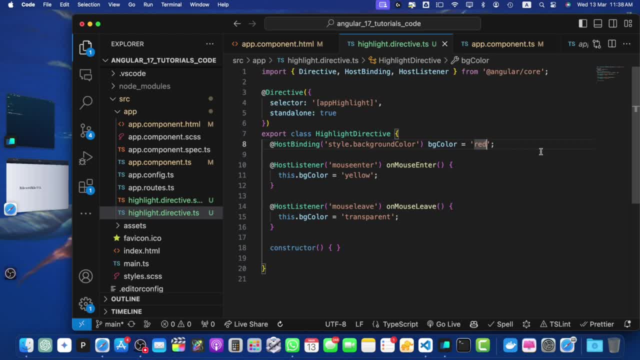 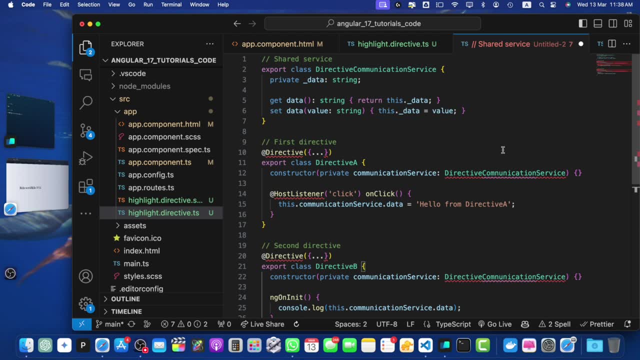 allows directives to share data and functionality via common service. so this is an example of how you might use a service to communicate between directives, you can see. so this is just to give you the imagination of how we will use in the real world. so this, imagine, this is a service. this would 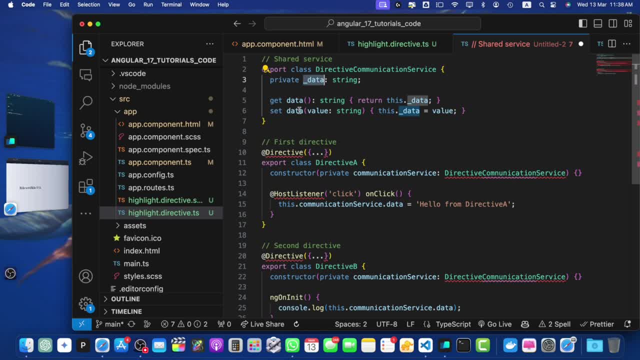 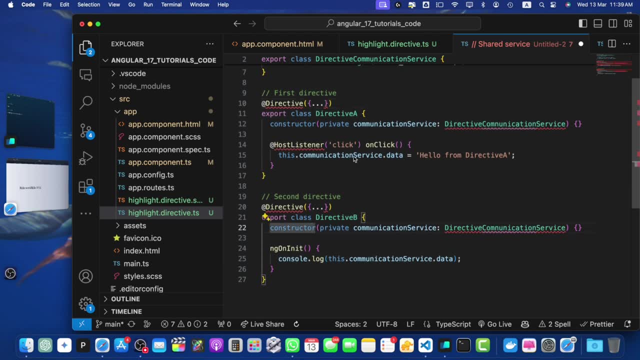 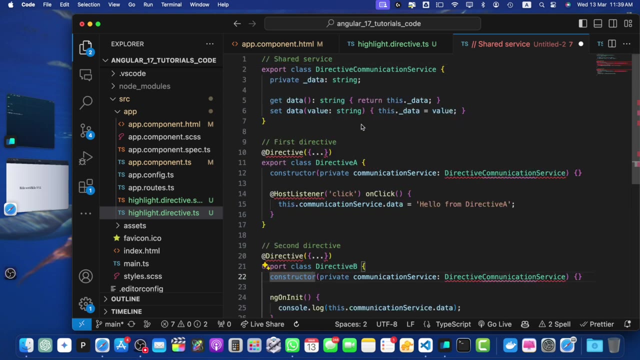 be in a separate file and we have the data and getter and setter, then we have a directive, and so this is a first directive and this is our second directive here. directive a sets the value on directive communication service when its host element is clicked. directive B can then read that value when. 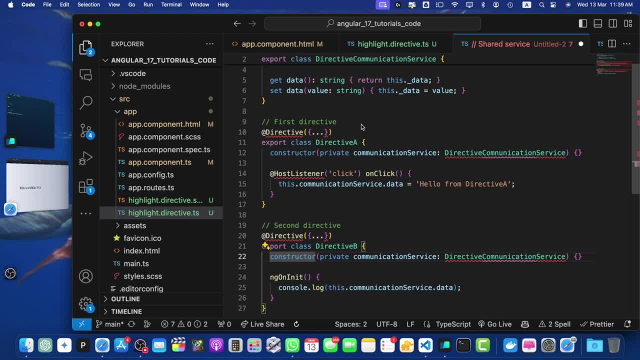 initializes when it initializes. so this is just one pattern for directive communications. the possibilities are endless. next, let's talk about creating your own structural directives. remember, structural directives are the ones that modify the Dome itself by adding and removing or replacing the elements. creating a structural directive involves working with angular's template syntax, so the key thing to understand is the 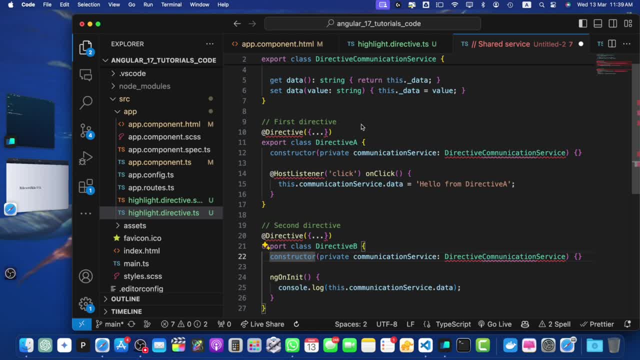 Asterix syntax. that star before the directive name- under the hood the star is Asterix- is a shorthand for using an ng template element. angular will wrap your host element in an ng template and then give directive full control over when and how that template is instantiated. so let's create an. 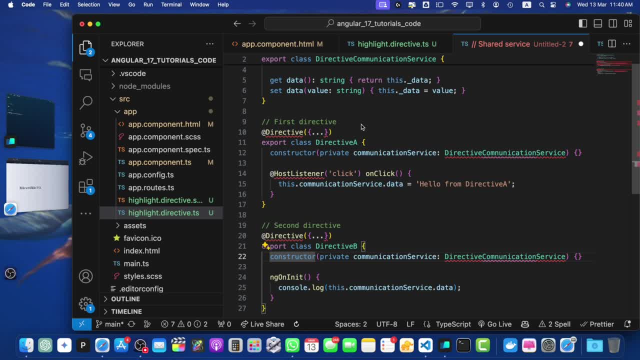 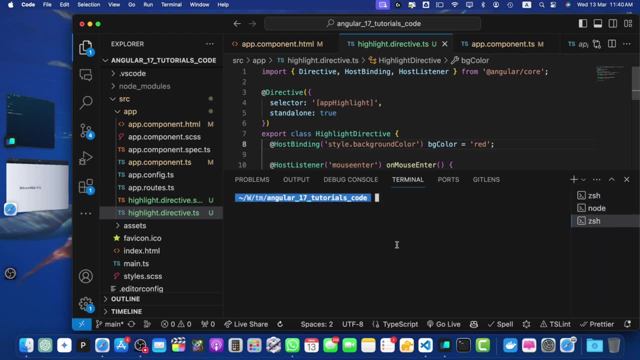 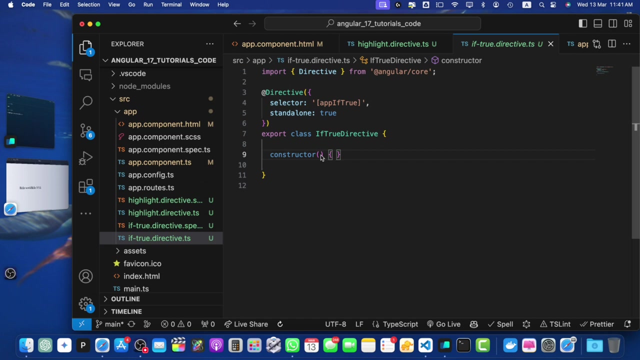 example of custom structural directive that conditionally renders its content based on a boolean input. so I am going to create a new directive by running the command g, generate directive, and I will give it name. if true, press enter. okay, the directive has been created and now I will. in the constructor I will inject some services like private template ref. template ref. make sure. 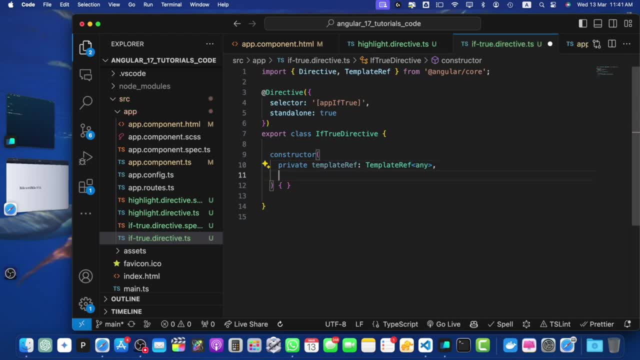 to import it from the angular core, and then we have the private view container and import the view container ref as well. after that, I will create an input like this: make sure to import it from the angular core as well and give it a setter app, if true, and we will define a function here that will receive the condition in this in this. 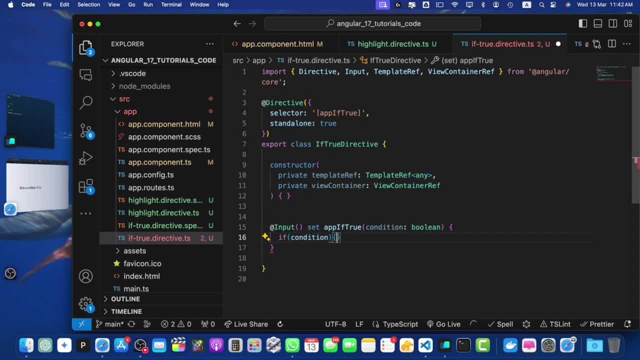 way and then I will check. if condition is true, then we will add this dot- view container, dot create embedded view and pass the this dot template ref in the. else we will call the clear function on the view container. so in this directive we inject the template ref. 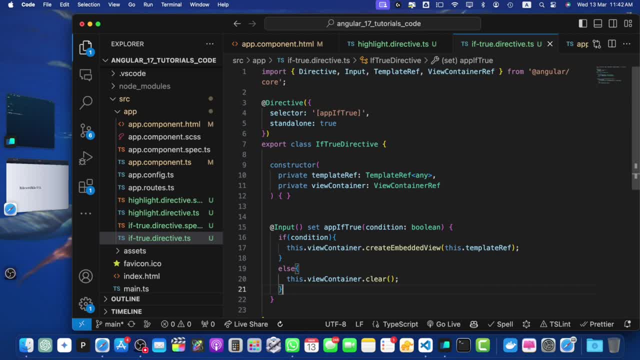 which represents the content of the host element, and the view container ref, which represents the container where we can in instantiate the template. the input setter gets called when the app. if it's true, we instantiate the template using the create embedded view. if it's false, we clear the container. 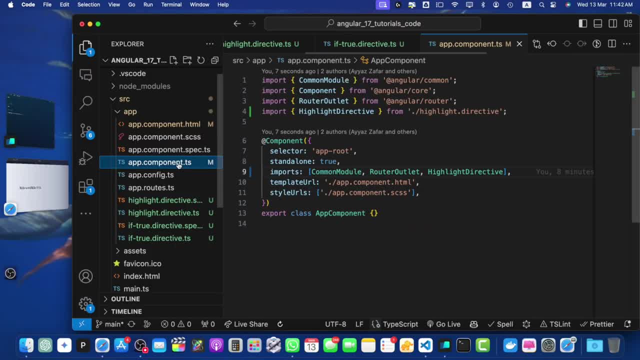 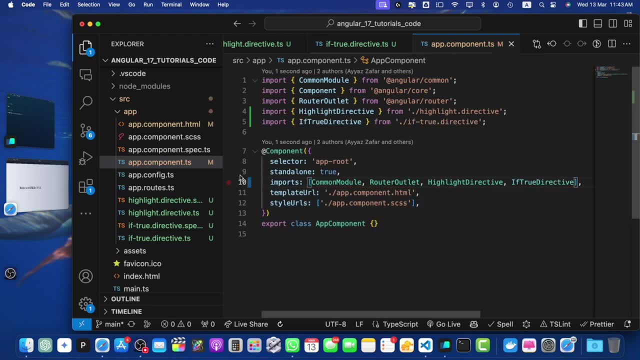 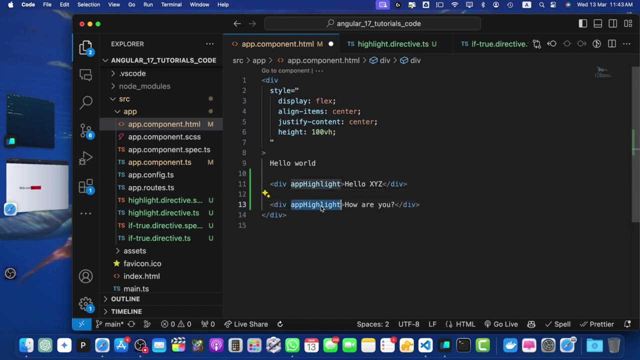 effectively removing the content. so let's use this directive for that. in the imports in the app and now in the html, I will add another div and here I will use app. you can see it is available in the suggestion, so I will select this and here I will pass the condition. so, for example, if there 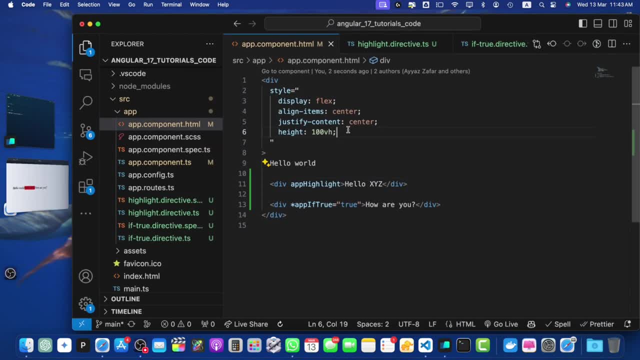 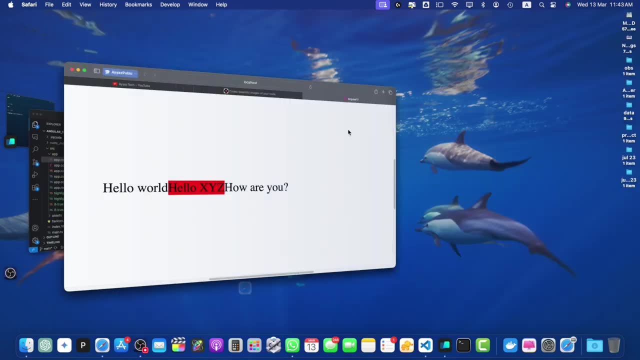 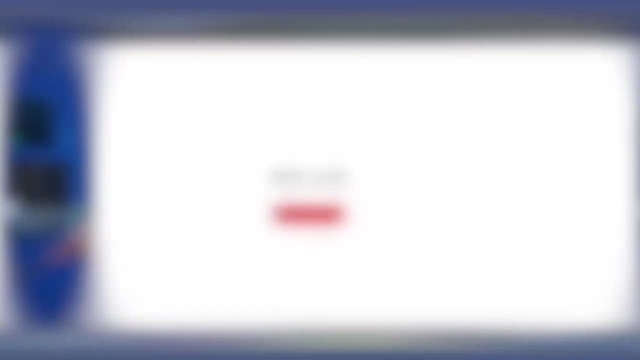 is true, then it would be visible. let me fix the alignment here in the flex, flex direction column and gap of 20 pixels. all right, so you can see that this is visible. but if I pass false here, then it will not be visible. so you can also use a dynamic variable from your. 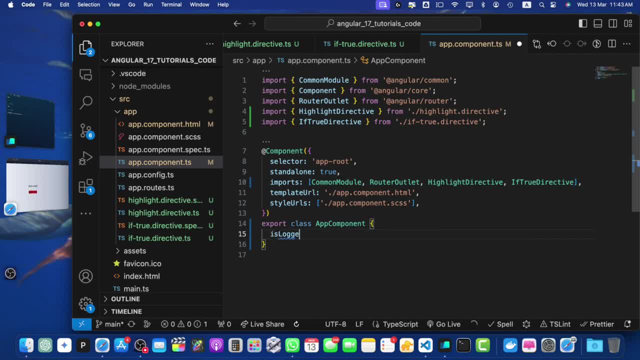 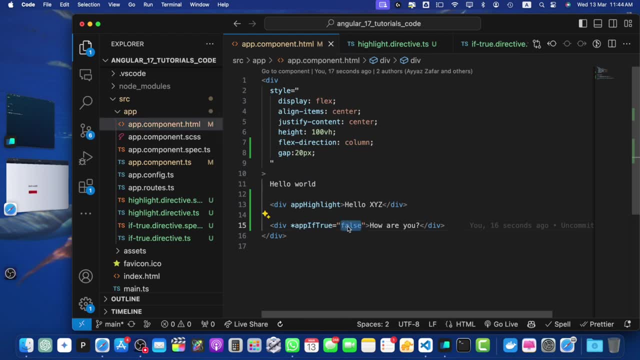 TS file like is logged in is equal to false and use that variable here instead. but for that here I will add: is logged in in this double quotes and now you can see it is not visible. but if you go back here and set it to true then it would be visible again. 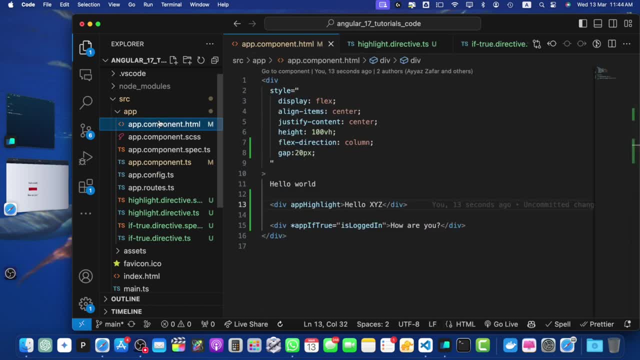 so the structural directives can also provide a context to their templates. so this lets you pass data into the template that it can use during rendering. to provide context, you use the set method on view container ref and pass in a context object. the template can then access this context using the template variables. so for that we have to change this line of code. 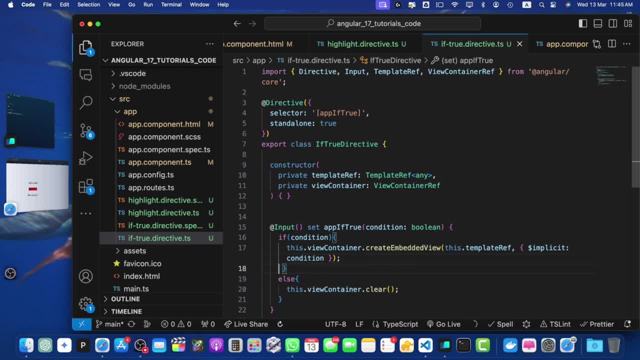 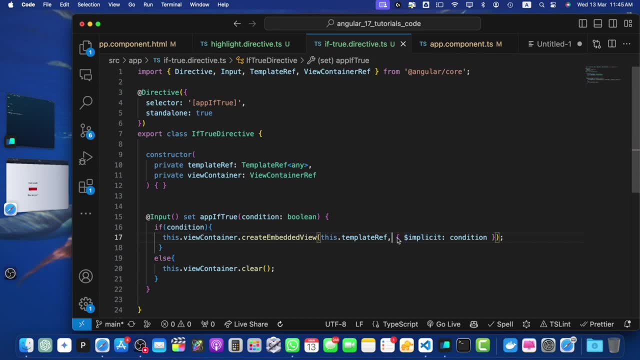 in this in this way. so this time you can see, we are passing this template ref and we are also passing a second parameter, that is an object, with the implicit condition. okay, so in this version, the, we pass the object as the context when creating the embedded view. this makes the 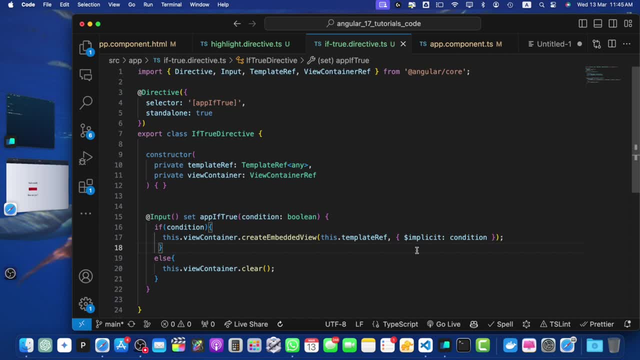 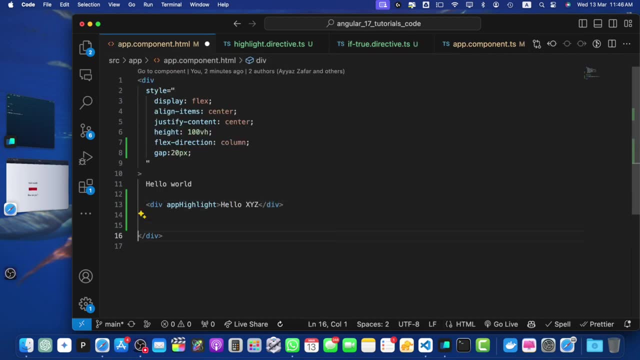 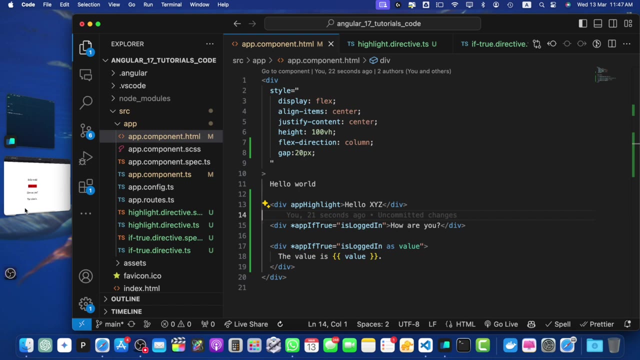 value of condition available in the template as an implicit variable, so you can use it in your template like this. and here let's add this: okay, the as value syntax assigns the implicit context variable to a template variable named value, which can then be used in interpolation or other template expressions. creating custom structural directives gives you a 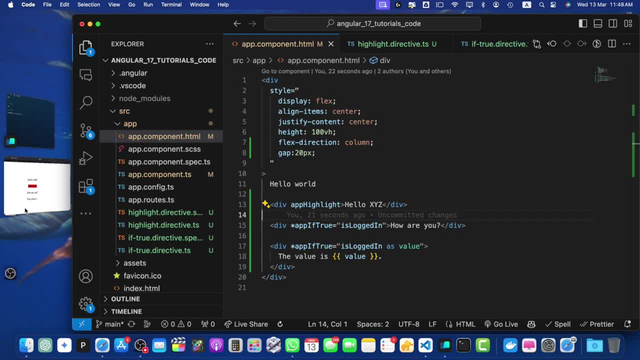 lot of control over rendering of your templates. with the static a star, syntax, template ref, view, container ref and template context, you have the tools you need to create your own structural directives that can manipulate the dome in powerful ways. that wraps up our deep dive into advanced directive techniques. with these, 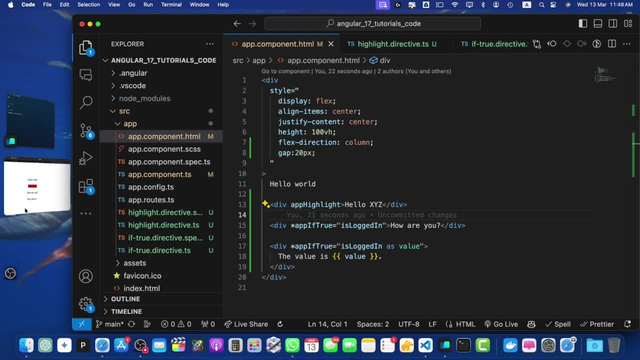 tools in your belt, you are ready to create some truly impressive and reusable angle directives. the only limit is your imagination. now we will cover some best practices for creating directives that are maintainable, performant and well tested, so let's dive in first up. let's talk about 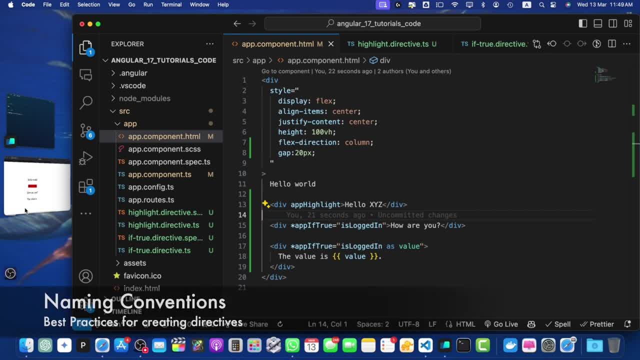 naming conventions. while it might seem like a small detail, having a consistent naming scheme for your directives can make a big difference in the maintainability of your code base, especially as it grows. so here are some guidelines to follow. first one is: use a consistent prefix for your 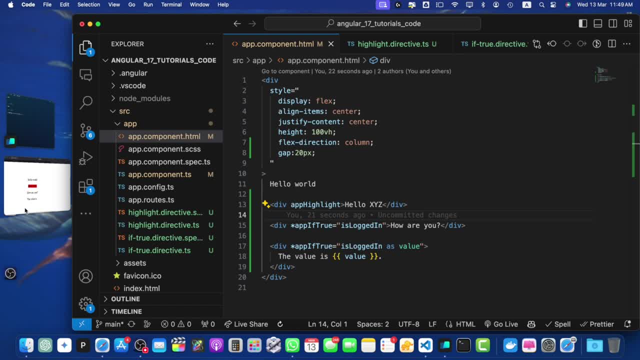 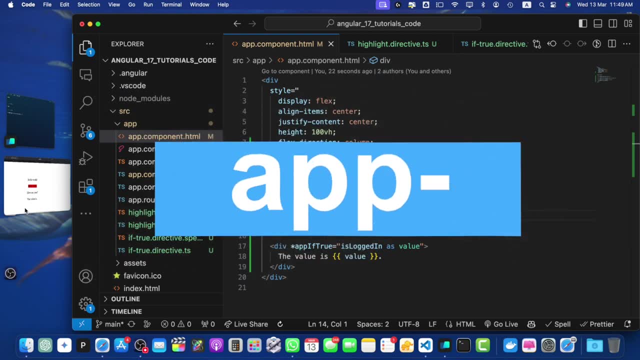 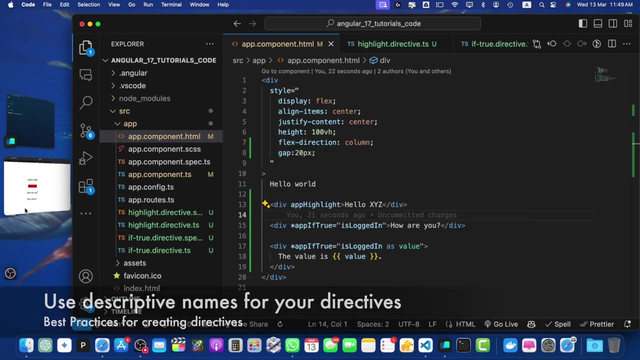 directives. the angular style guide recommends using a prefix that identifies your app or organization, like app dash. this helps avoid naming collision, so you will be able to check the code with the third party libraries. use descriptive names for your directives. next guideline is to use descriptive names for your directives. the name should clearly: 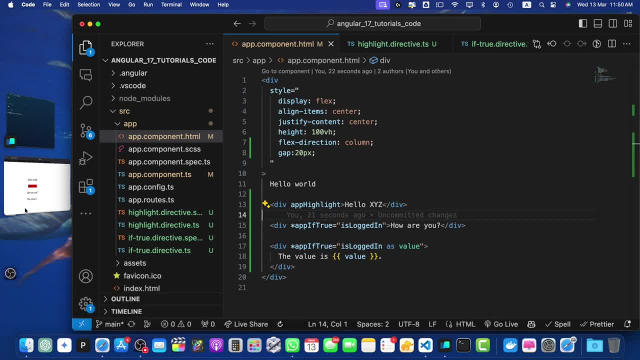 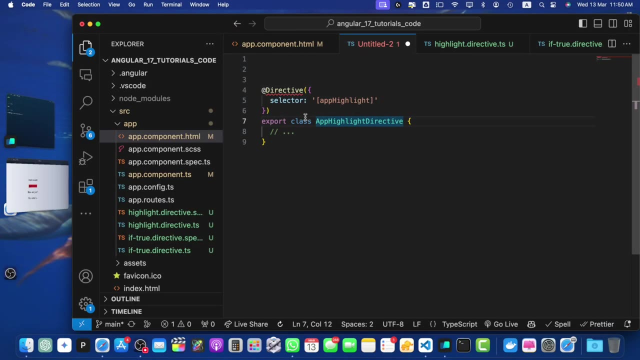 indicate what the directive does. for example, app highlight is better than just app color. next one is using camel case for the directives selector and pascal case for directives class name. this is consistent with angular's general naming convention, And a well-named directive might look like this: 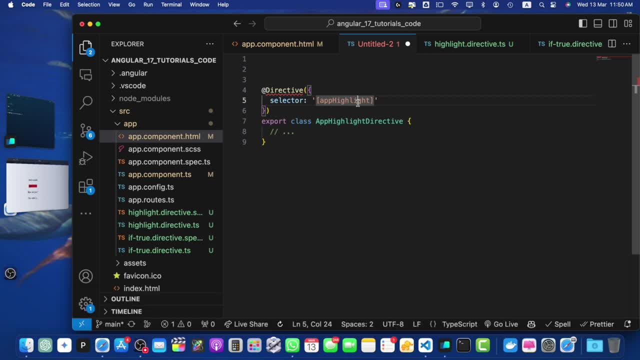 Next, let's talk about performance. Directives can have a big impact on your application's performance, especially if they perform a lot of DOM manipulation. So here are few tips for optimizing directive performance. First one is: minimize DOM manipulation. Accessing and modifying DOM is expensive, so try to batch your update and avoid unnecessary. 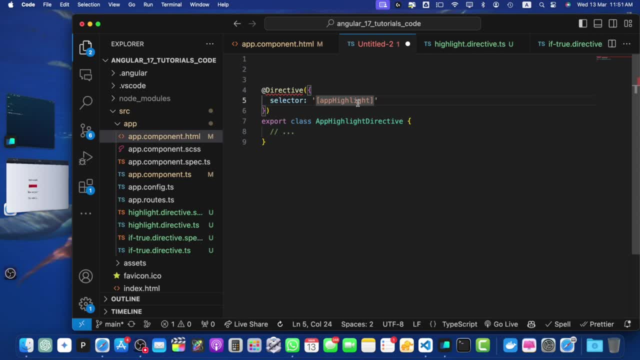 changes. Use host binding to modify the element properties directly instead of using the render to. when possible, Use efficient change detection strategies. If your directive's data doesn't change, often consider using the onPush change detection strategy. This tells Angular to only check for the changes when the directive's inputs change rather. 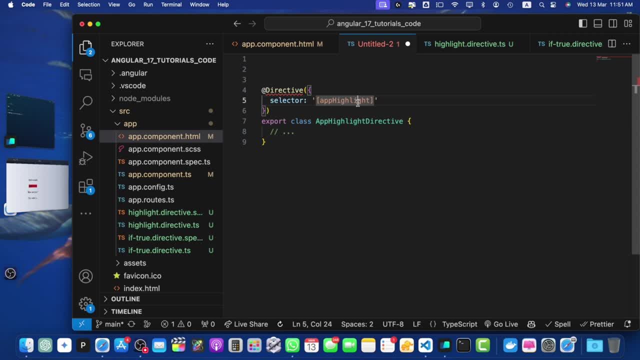 than on every change detection cycle. Just be careful not to mutate your inputs. So here is an example. Here is an example of directive that uses these techniques. In this directive, we only update the content when the data input changes and we use the 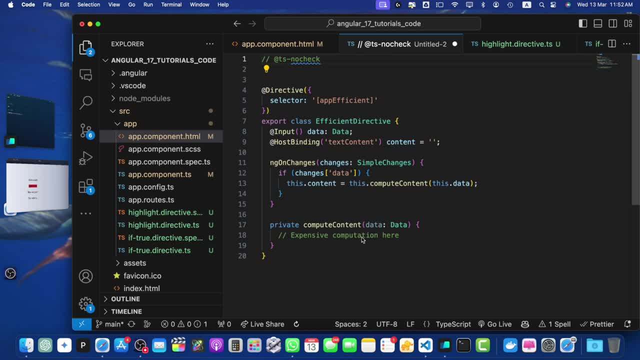 host binding to set the text content directly, avoiding unnecessary DOM manipulation. Finally, let's talk about testing. Just like any other part of your Angular application, your directives should be thoroughly tested. Angular's testbed makes it easy to write unit tests for directives. 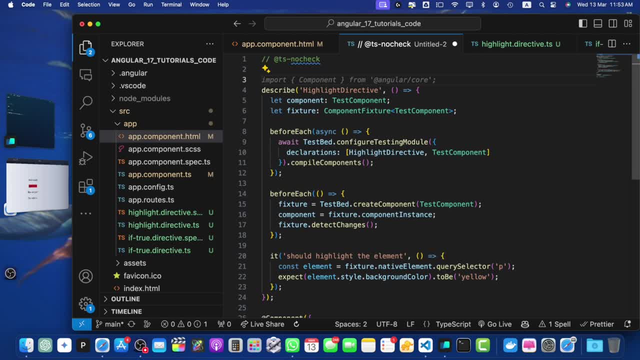 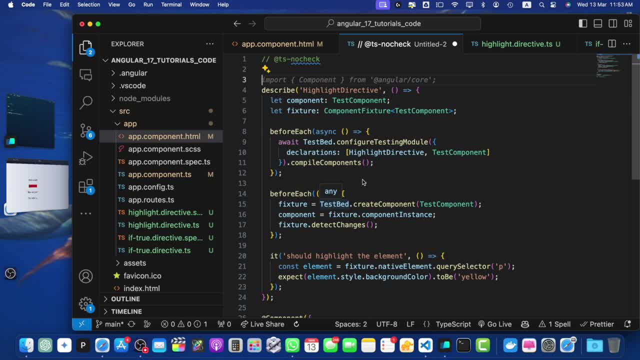 In this test we create a test component that uses the directive. Then we assert that the directive has had the expected effect on the host element. If your directive has dependencies, you can mock them using Angular's dependency injection system. Just provide the mock in the testing module. 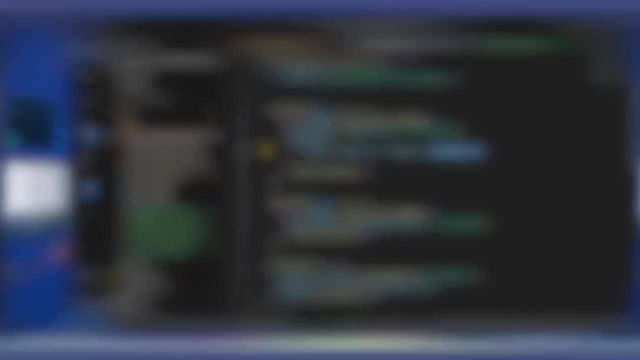 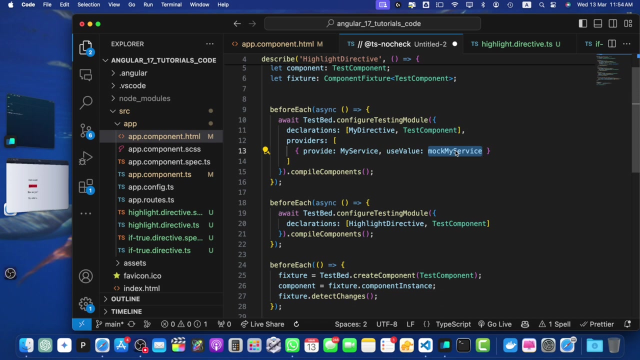 Like this. We have provided the mock, So this allows you to test your directive in isolation from its dependencies. And that's it. By following these best practices- using clear naming, optimizing for performance and writing thorough tests- you can create directives that are a joy to use and maintain. 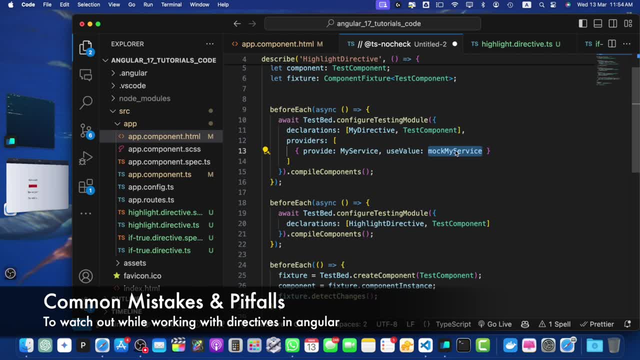 Now we will cover some common mistakes and pitfalls to watch out for when working with directives in Angular. First and foremost, One of the most common mistakes is forgetting to write directives. The most common mistake is forgetting to declare your directives in the module or component. 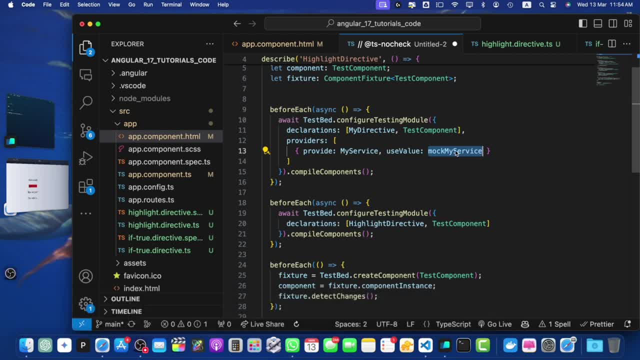 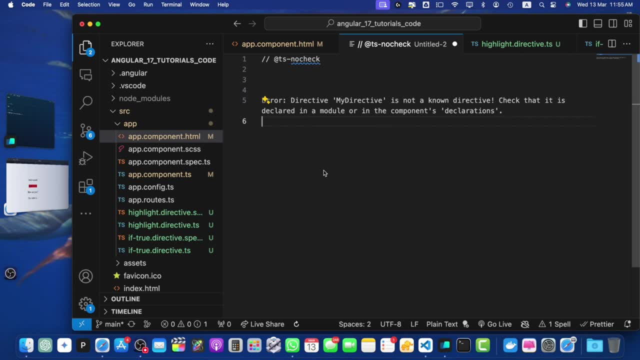 where you want to use them. If you forget to do this, Angular won't recognize your directive and you will get an error in the console Like this. To avoid this, make sure to always add your directive to the declarations array in the module or in the imports array of the component if you are using standalone components. 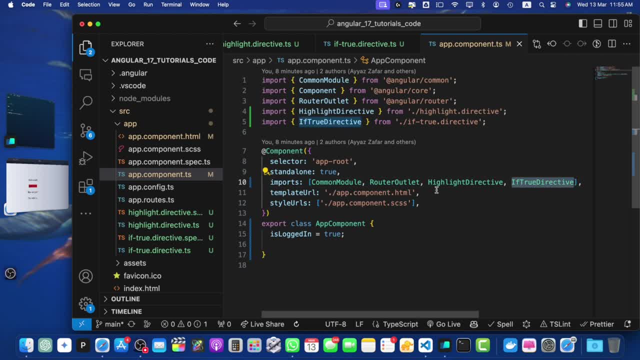 Like we did here. We added this. We added these directives in the imports array because my component was standalone. But if you are not using standalone components but you are using modules, you can declare these directive components in your relevant module. Another common pitfall is incorrect usage of the input and output decorators. 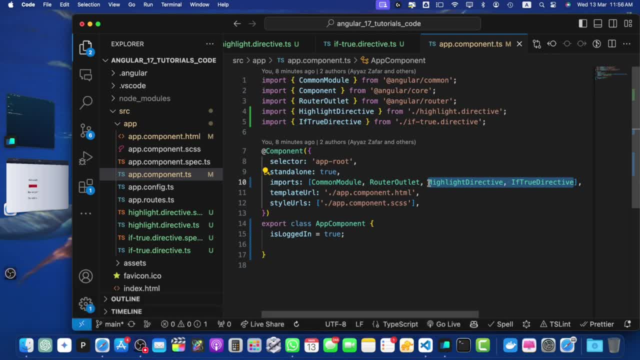 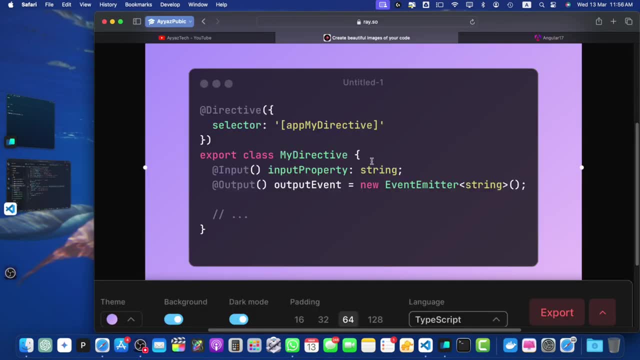 Remember, input is for properties- that you want to pass data into your directives- and output is for events. Your directives are for events. So here is an example of correct usage. A mistake I often see is people forgetting to add the decorator or using input for an. 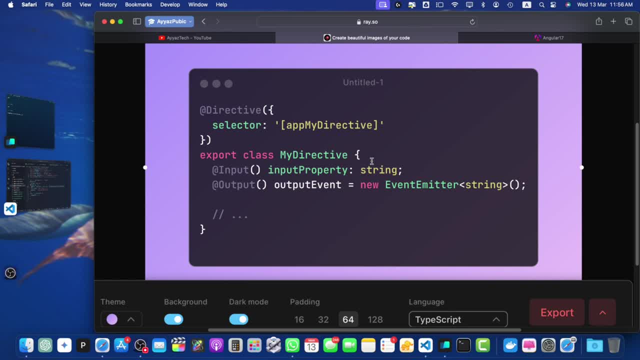 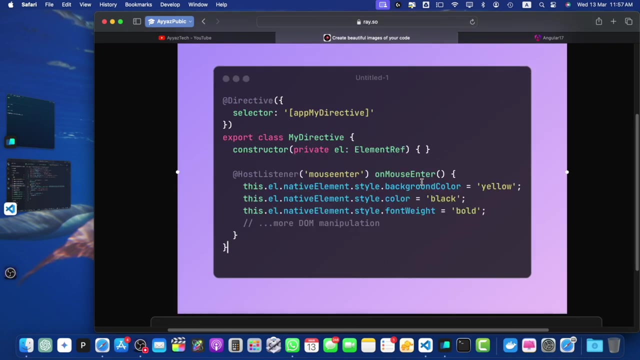 output property or vice versa. Double check that you are using the correct decorator for your purpose. Performance is another key consideration when creating directives. Excessive DOM manipulation can lead to performance issues, especially in directives that are used frequently. So here is an example of excessive DOM manipulation. 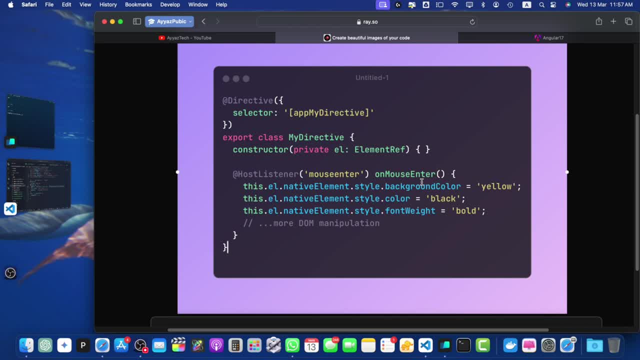 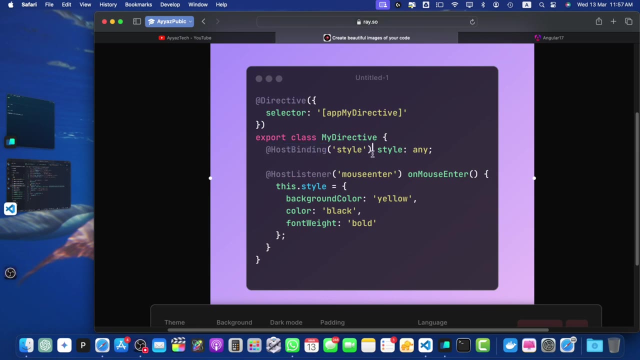 So here is an example of excessive DOM manipulation. To mitigate this, try to use host binding instead of direct manipulation when possible. Batch your updates and avoid unnecessary updates like this. in my screen You can see I have used the host binding and now, on mouse enter, we are accessing that style. 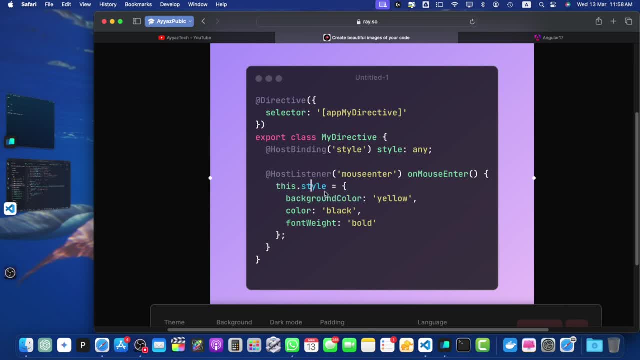 from the host, binding from the host, and we are updating all of the styles all together in one go. So, finally, let's talk about the host binding. Let's talk about debugging and troubleshooting directive issues If your directive isn't working as expected or you are seeing errors in the console. here, 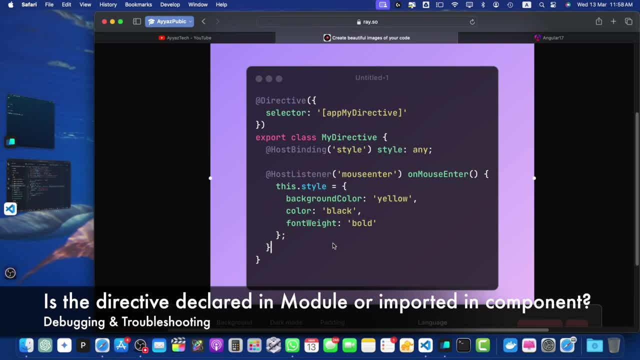 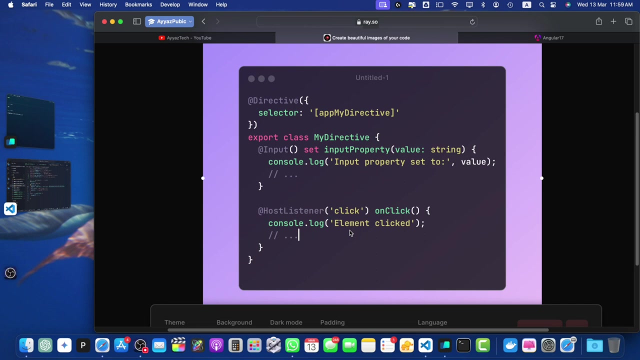 are few things to check. First one: is the directive declared in the module or imported in the standalone component? Is the selector correct? Are the input and output decorators used correctly? Can you track the flow of data with consolelog statements? Here is an example of debugging with the consolelog statements. 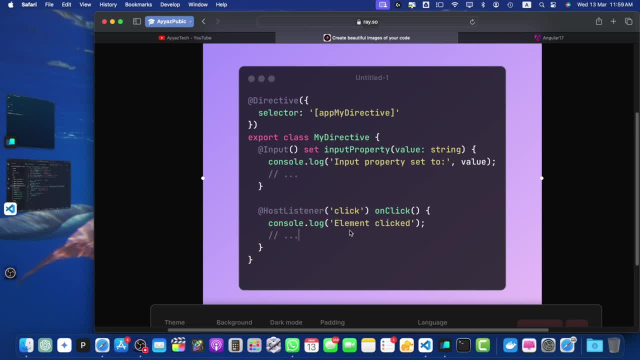 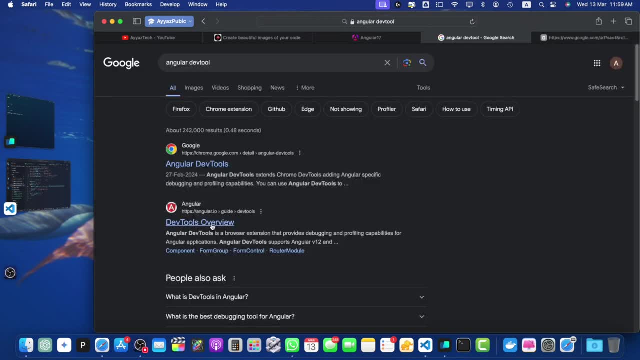 You can also use the Angular dev tools for debugging directives. They provide a lot of useful information and insights. So this is the Angular dev tool that you can see. it is also mentioned in their documentation as well, So you can review it and follow it. 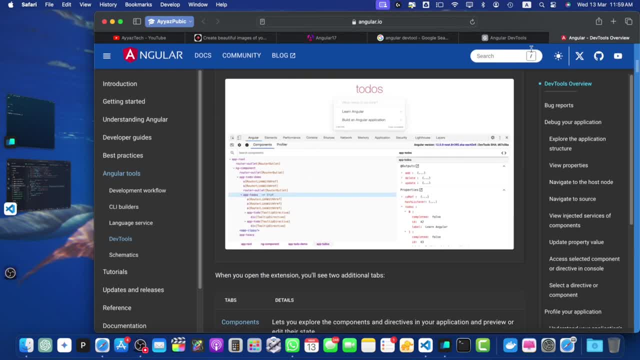 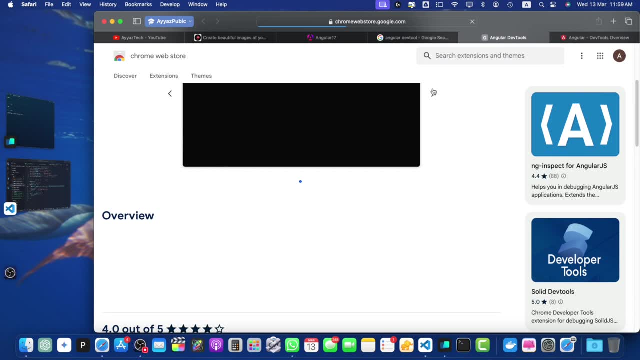 They have shown you the example how to use it, and it is very convenient and powerful. So this is the Chrome extension that you can install. So here is the Chrome extension that you can install And you can start using it. So this is the official extension by the Angular. 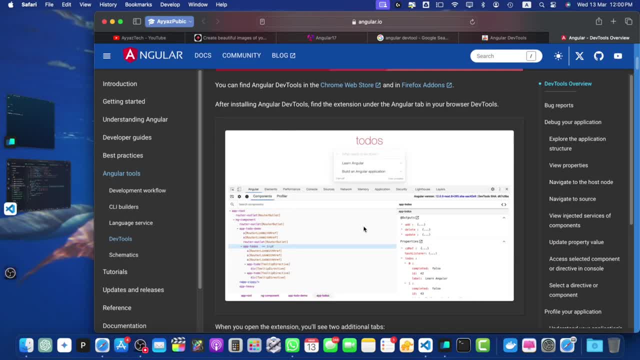 Now let's wrap up with our conclusion. In this tutorial, we have covered a lot of ground and we have learned what directives are and why they are important. in Angular, We have explored the three types of directives: components, attribute directives and structural directives. 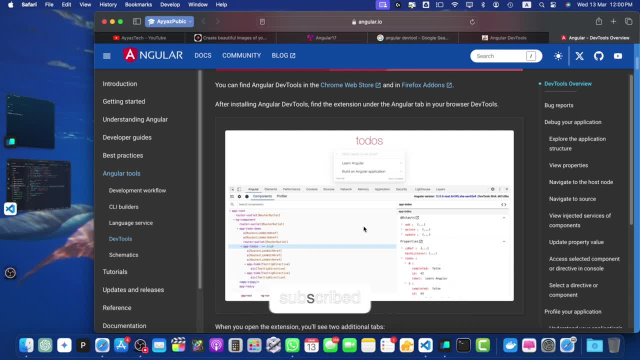 We have seen how to create our own directive. We have seen how to create our own custom attribute and structural directives, And we have discussed the best practices for directive creation and usage. But learning about directives is just the beginning. The best way to truly master directives is through practice and experiments.